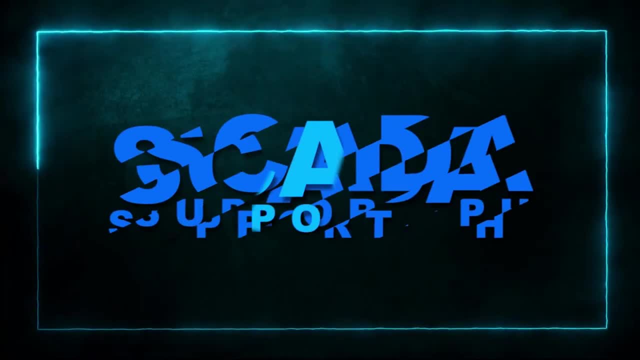 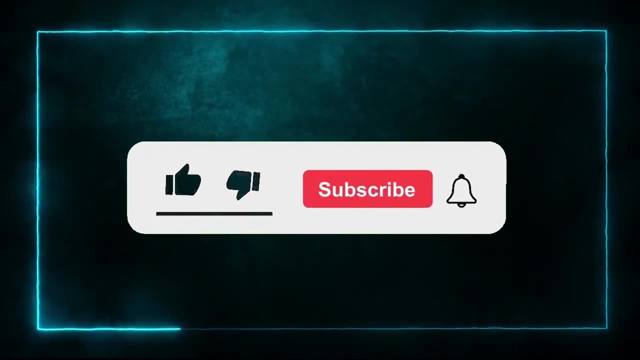 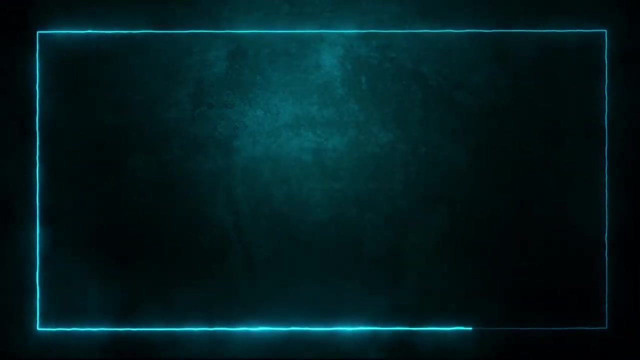 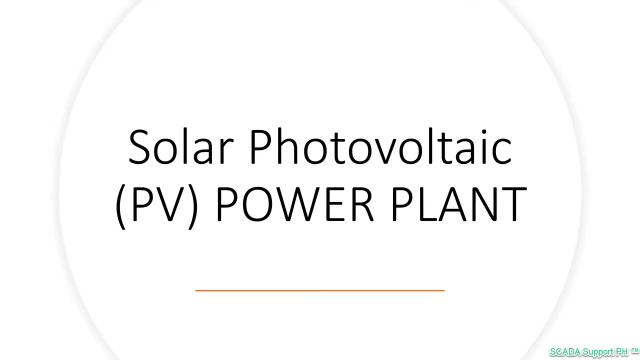 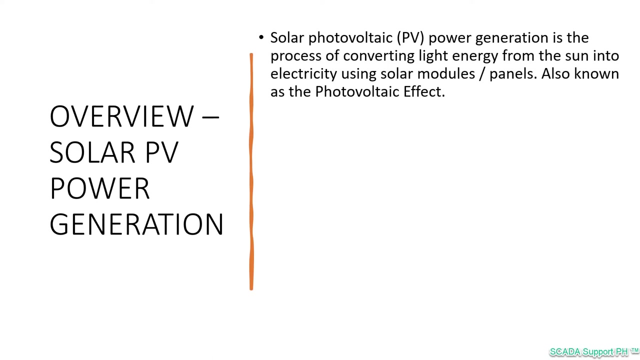 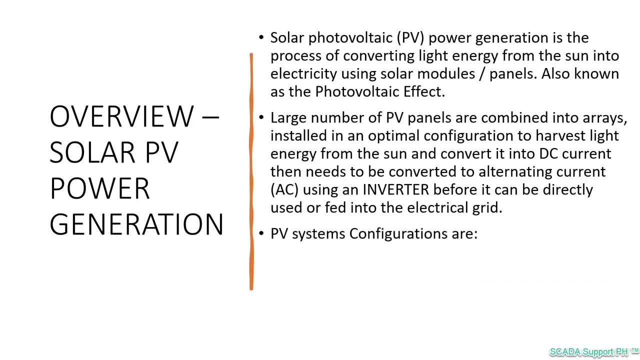 In this video, we will discuss about solar photovoltaic power plant. As an overview, solar power generation is the process of converting light energy from the sun into electricity using solar modules, and this is also known as the photovoltaic effect. PV systems can also be installed in grid-connected or off-grid configurations. 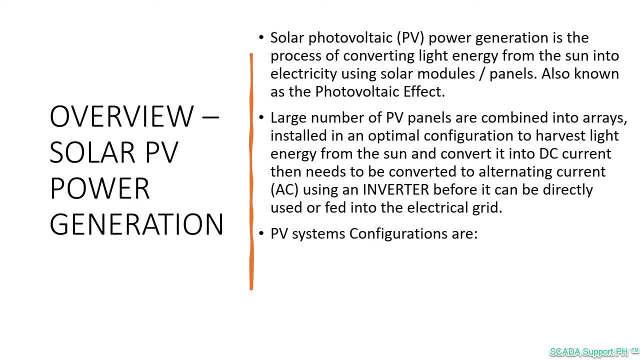 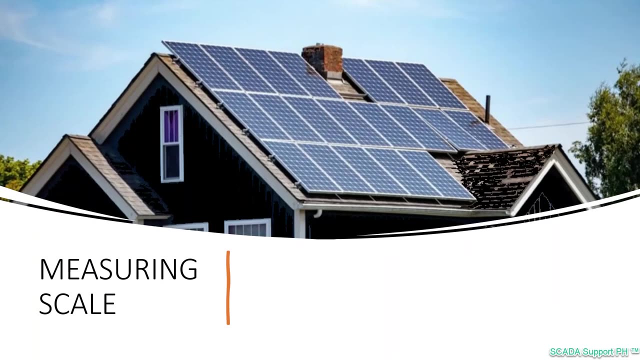 Grid-connected configuration is commonly used because it is easier to install and less expensive compared to off-grid PV systems, which mostly rely on batteries. In terms of measurement, there is no commonly accepted definition as to what size constitutes a PV system. Don't believe it. 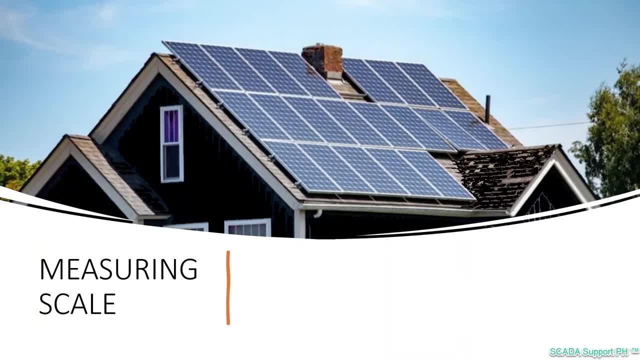 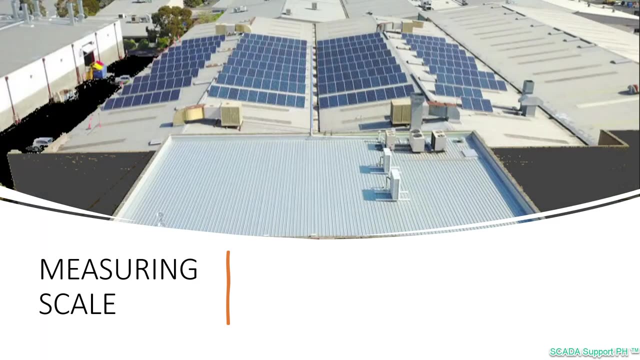 Quick online search reveals a wide range of definitions for each. For a given example, residential grid-connected PV systems are rated less than 20 kW. On the commercial side, commercial systems has an output power range from 20 kW to 1 MW and are considered as a form of distributed generation. 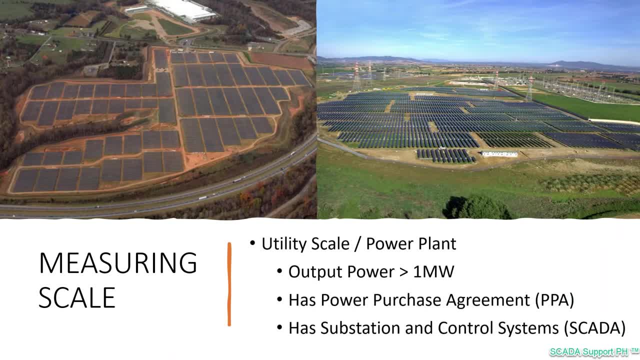 When it comes to utility scale, we are looking at systems that has an output power that is more than 1 MW. A utility-scale solar facility is one which generates solar power and feeds it into the grid, supplying a utility with energy. Virtually every utility-scale solar facility has a Power Purchase Agreement with the utility. 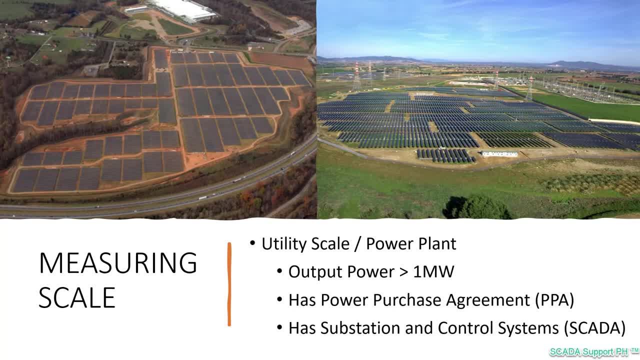 guaranteeing a market for its energy for a fixed term of time. The only way to sell solar power to a utility is through a net metering structure, which generally power is used on-site and excess power is fed into the grid. This is a good example of a grid-connected PV system. 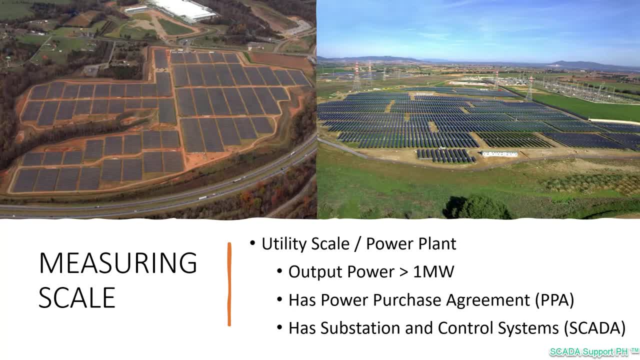 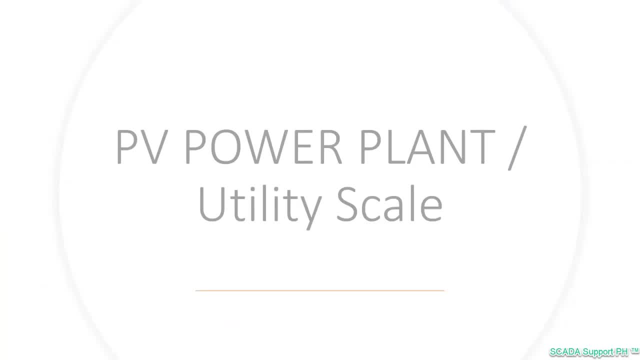 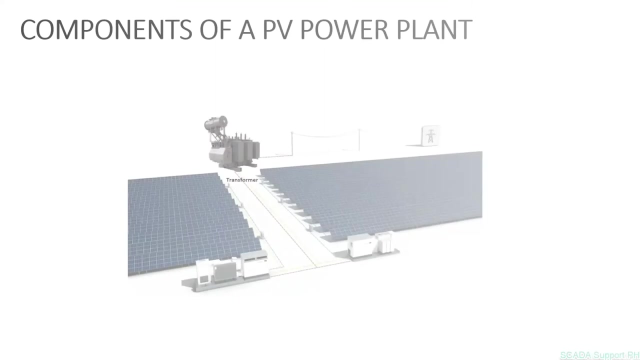 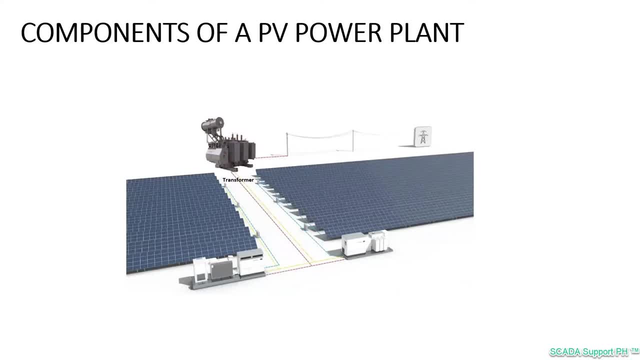 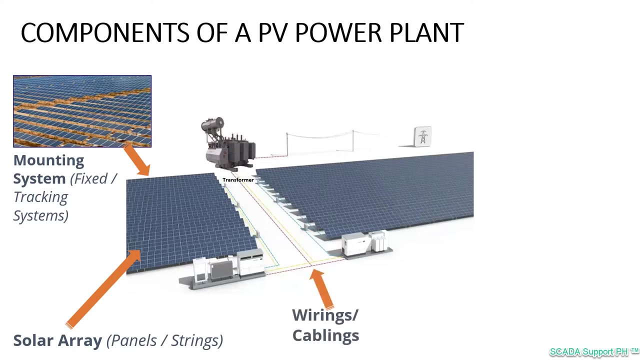 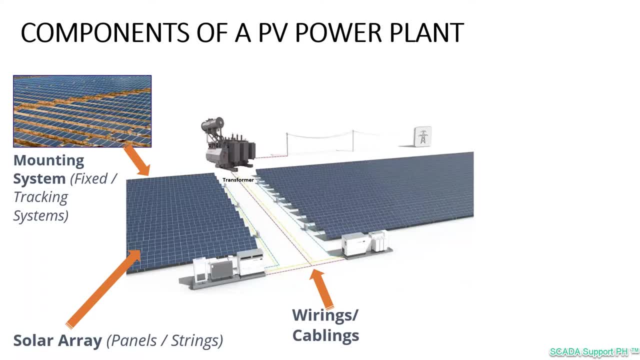 Wirings and cabling, which are electrical wirings that can be passed on to the plan to be Narrator and simply analyzed in depth. That can be the power plant, power plant, energy socket soldering facility, power plant and electricity. 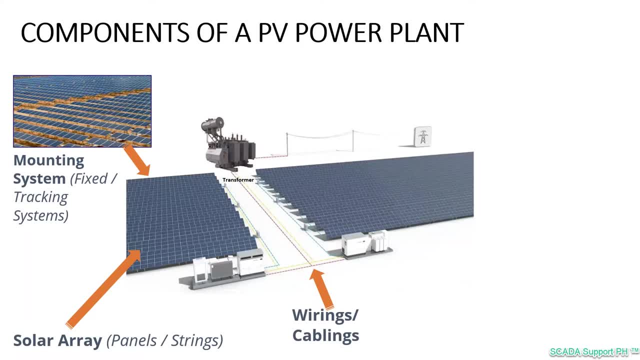 connects all your strings that runs from the array to the inverter, and you also have your cable links related to network and data communications. skids or pads is a set of assets or equipments that are geographically located in one single area. this would either include one or two inverters, meters, your low voltage and medium. 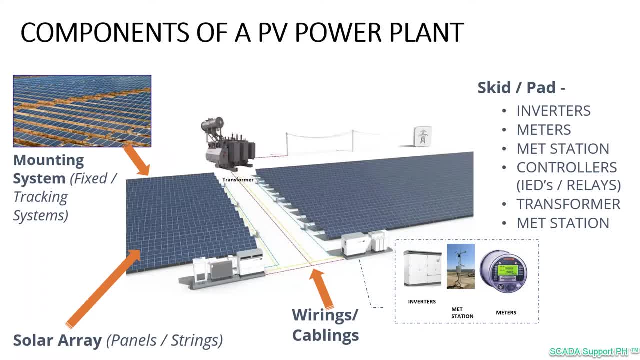 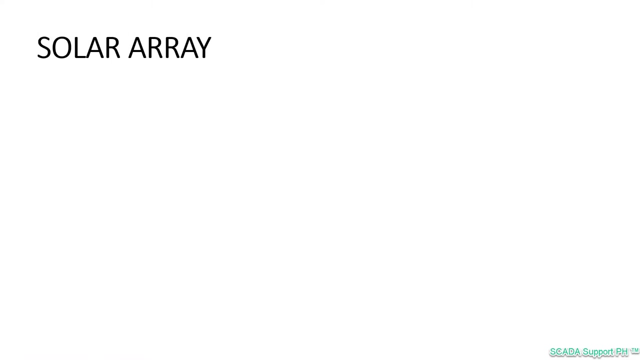 voltage transformers, and it depends on the system design, as well as your met station, and at the top you have your grid connection interface. this is collectively known and as your substation, where controls are being imposed as well as electricity, is exported into the grid network. let's discuss about solar array. solar array- 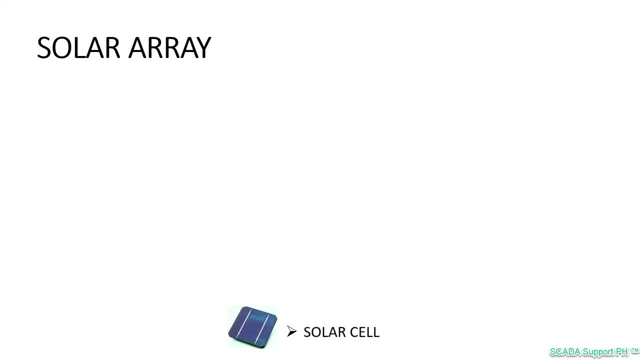 would start from single solar cell. so a solar cell or a PV cell is basically a piece of silicon. this was manufactured to convert the energy of light directly into the grid network into electricity through the photovoltaic effect. Next is the solar module, which is typically 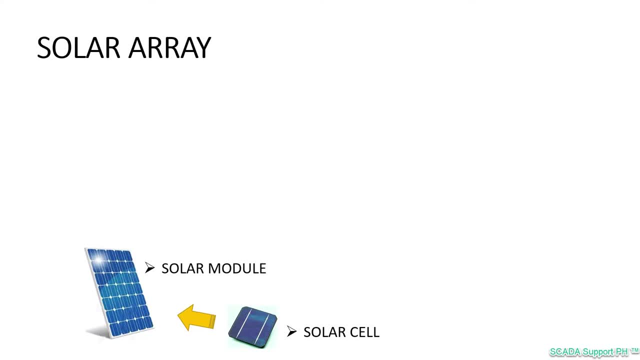 composed of 60 to 70 cells in a single assembly. This is a self-contained unit which has leads coming out of it, And modules can be connected together in a series to produce a string of modules. When connected in series, the voltage increases. 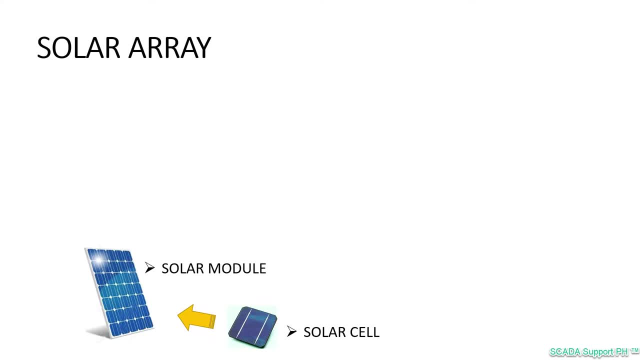 And, on the other hand, strings of modules connected in parallel increases the output current. Please take note that a module is not a panel. A panel is an assembly of multiple modules combined together to form a single unit. Combining multiple panels becomes an array. 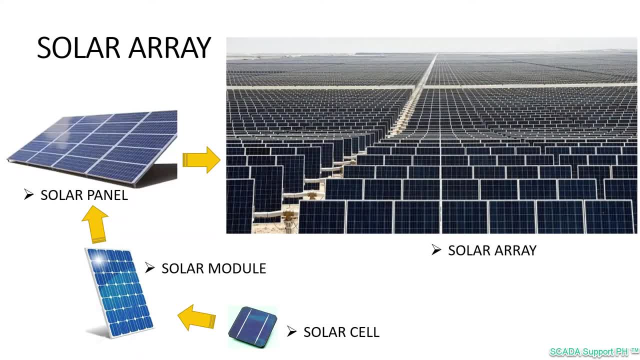 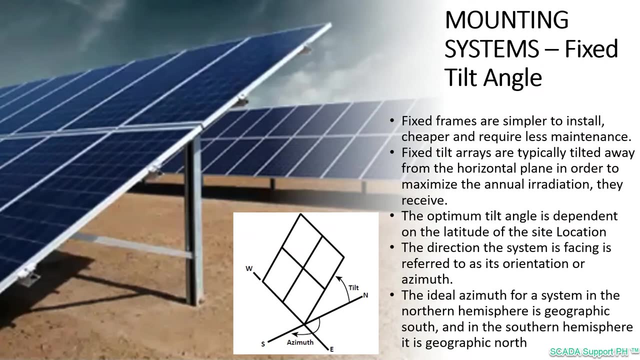 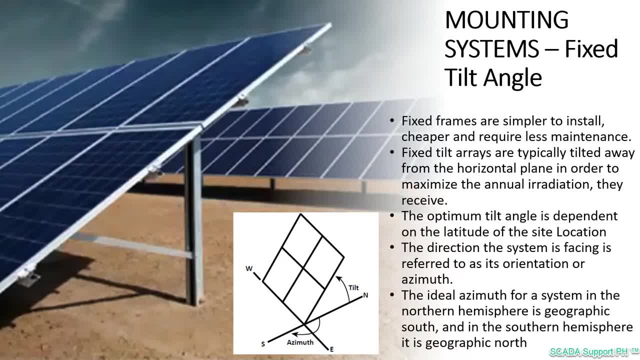 And this is a very important point, And this is an interesting point- The models are for such an array of different meters due to the leader of the uppermost layer, And the levitation unit has exactly the same welding Budduk as the optimize. 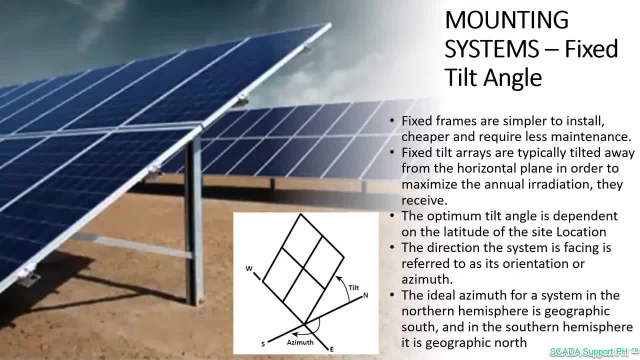 because all the inclinations have differentobs. Toliver project The into element across all the Turks in the up here, the optimal power production. The direction that the system is facing is referred to its orientation, or what we call azimuth. If the ideal azimuth for a 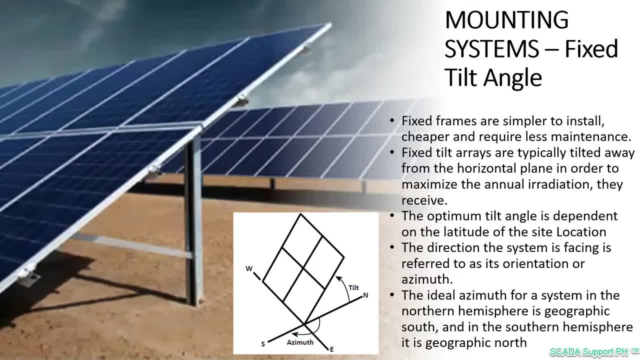 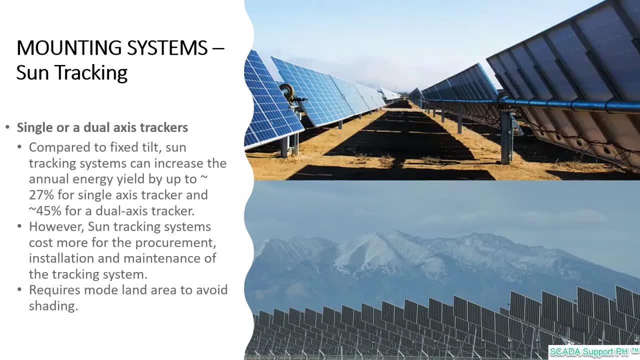 system in the northern hemisphere is your geographic south and in the southern hemisphere it is geographic north. Sun tracking systems, on the other hand, they may be single or dual axis tracker and these systems follow the Sun as it moves across the sky. These are: 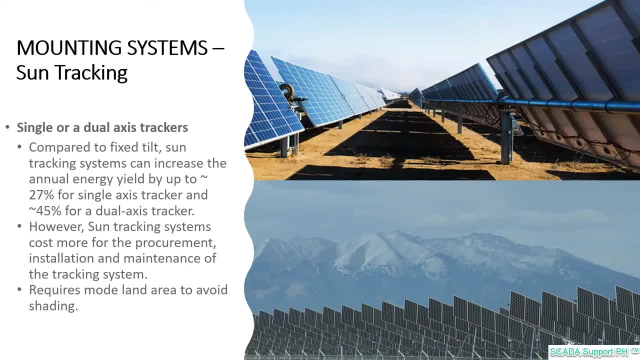 generally the only moving parts employed in a solar PV power plant. Axis trackers are used to optimize performance, as they allow for panels to track the Sun as it moves position throughout the day. However, sun tracking systems cost more in terms of procurement, installation and. 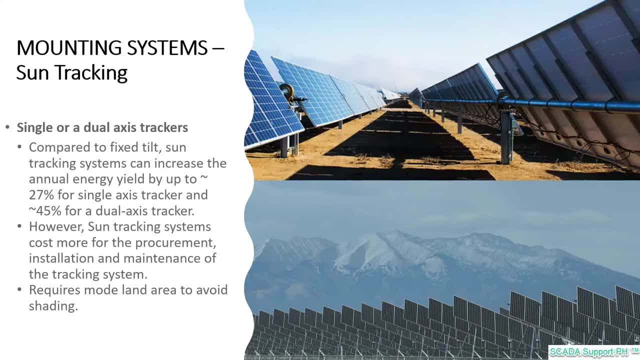 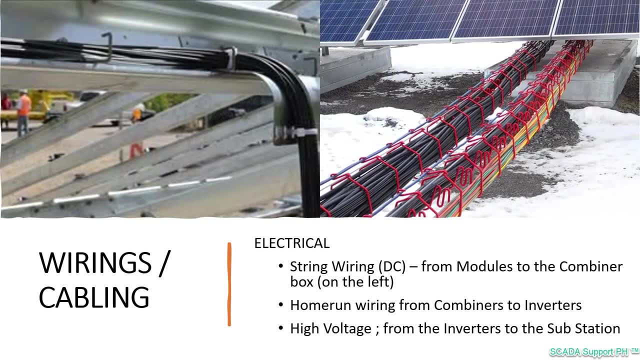 maintenance. When we look at the power plant overall, we can see different types of wiring. On this example, we have the electrical side that's going to carry the electricity. The lowest level of electrical wiring is the string level, Usually 10 to 25 modules within a 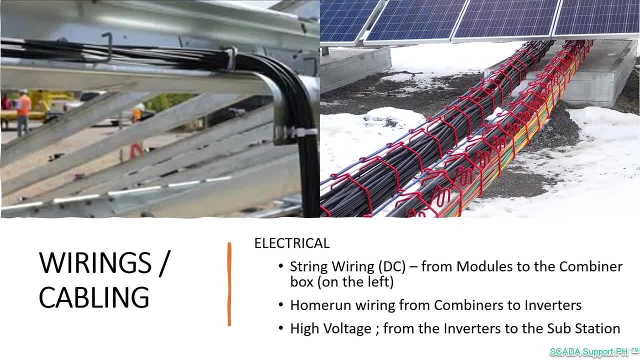 string and those wires from the modules are connected in series, meaning you have the same current. Then we'll bring all your strings together to a combiner box. Then we move the combined wires coming from multiple combiner boxes into a home-run wiring towards the dedicated inverter. that's the image on the right. 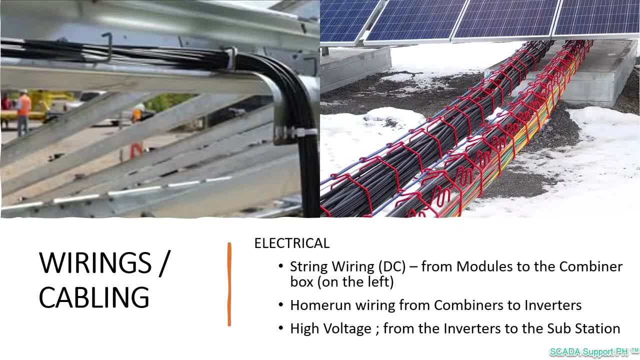 By design we are trying to minimize the amount of wire that we have it in the Array For us to minimize the resistance, as the more Ukaver tracks, the smaller the resistancekur Is. there's no Poly이고 hook structure. 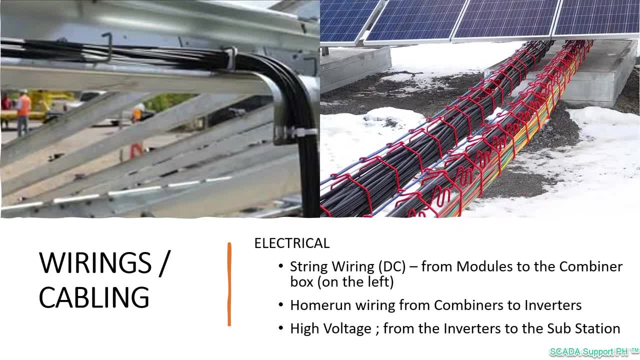 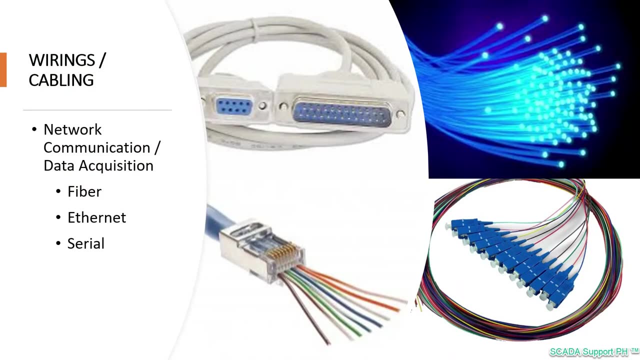 more resistance eventually leads to greater ohmic losses during operations. Wires coming off of the inverters to the substation: we consider them as high voltage. On the other hand, we also have cabling dedicated for our network communication or data acquisitions. Fiber optic cables are being used for its various data telecommunications. 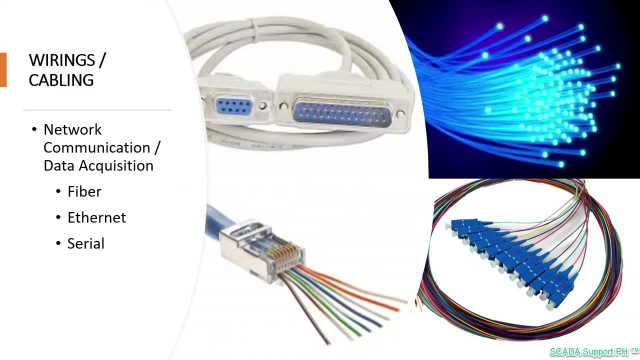 usage. These are usually installed between the SCADA communications panel on the SCAD and the substation where your SCADA servers are located. Since ethernet cables are limited to a maximum length of 100 meters, or around 230 feet, we consider them as high voltage Revenue-grade meters often use ethernet cables, while inverters 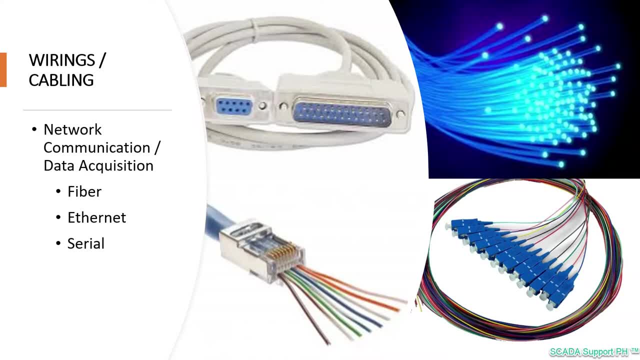 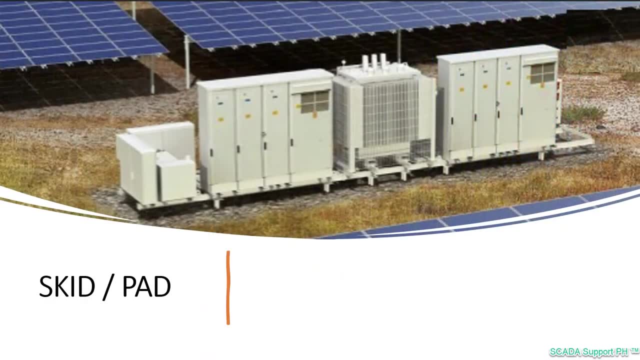 are more into serial communications using an RS-232 or an RS-485.. Here we have the SCID. A SCID is basically a set of assets or equipments that are geographically co-located in one system. It's composed of your inverters, meters, your low-voltage and medium-voltage transformers. 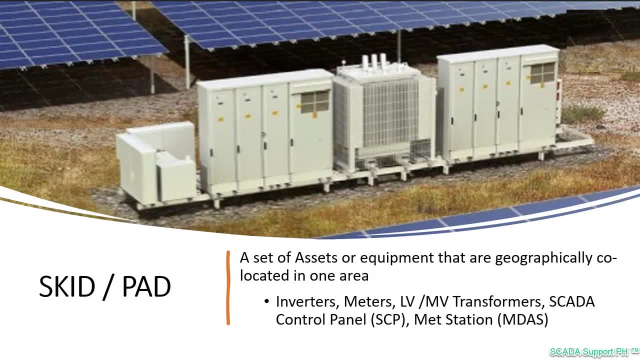 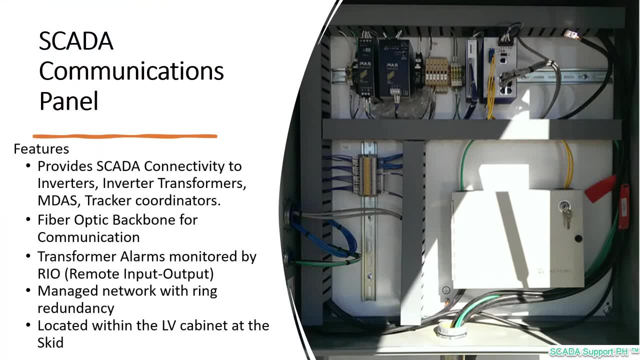 your SCP or SCADA control panel and your MET stations, or what we call MDAS, On a PV power plant. data communication and monitoring on the SCID level is very important, and this is where your SCADA communications panel comes in. This provides SCADA connectivity to your inverters. 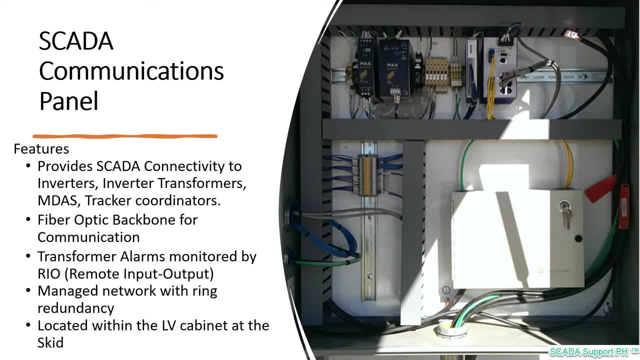 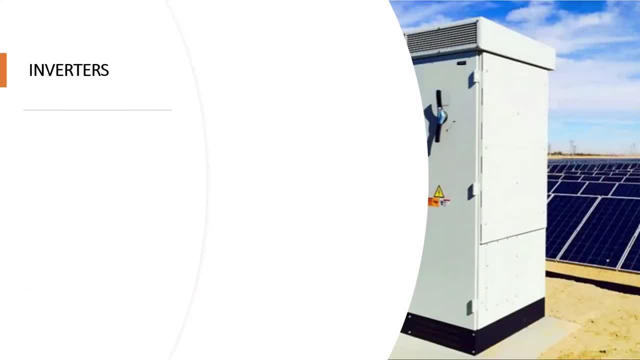 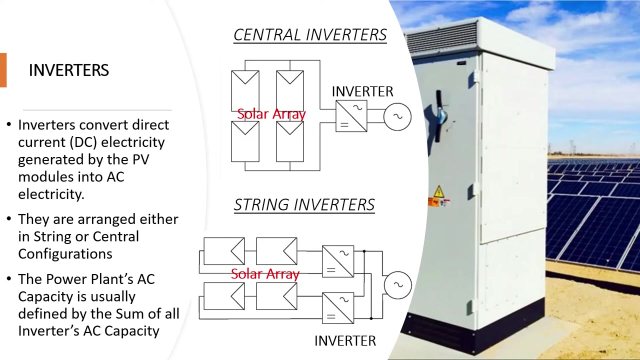 inverter transformers, MDAS and tracker coordinators. When we talk about inverters, Inverters- usually inverters- convert direct current or DC electricity PV modules into AC electricity. They are arranged either in string or central configurations. Central configuration inverters are considered to be more suitable for multi-megawatt plants, as it 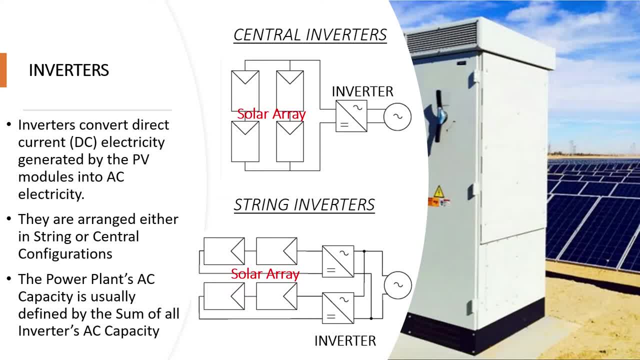 offers high reliability, simplicity and ease of installations. These are usually three phases and can include grid frequency transformers. Typical range for central inverters are from 50 kilowatts to 2 megawatts. On the other hand, string inverters enable 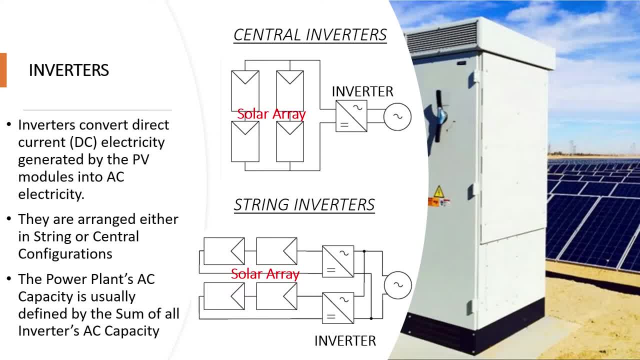 a control of the energy consumption of the plant. The control of the energy consumption of the plant is individual string maximum power point tracking and required less specialized maintenance skills. String configurations offer more design in terms of flexibility and are usually single phases. The output ranges of these string inverters are from 1 to 25 kilowatts. Please take note that inverters 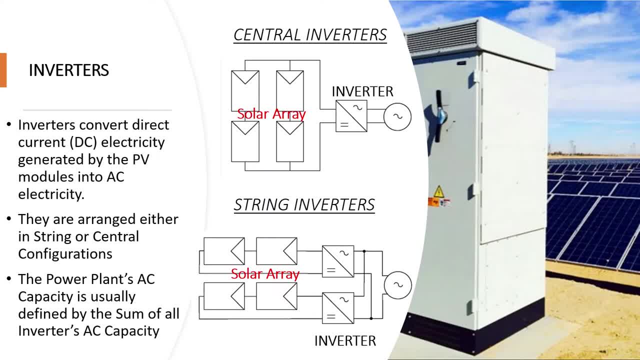 are active equipment, In other words, they are automated and can be used in all somewhere else for any use As well as waiting in line. The PV power plant AC capacity, or the amount of power it can produce, is usually being defined by the. 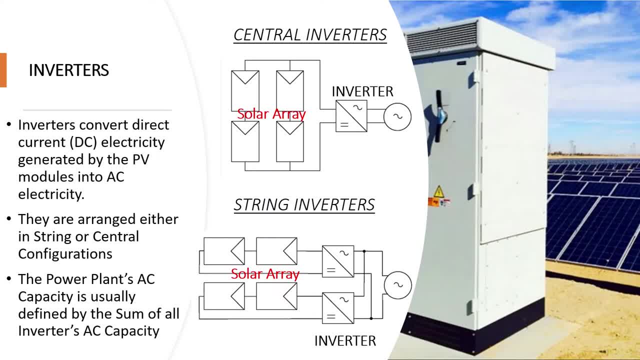 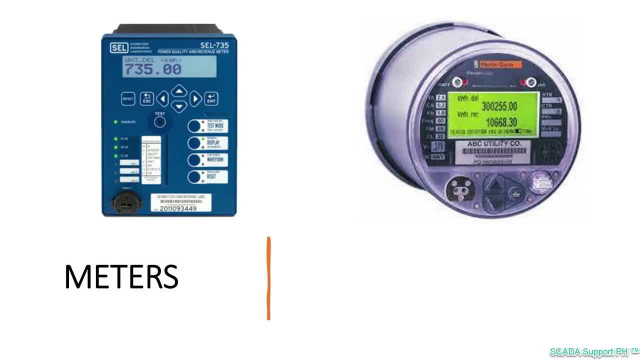 total or sum of all the inverters AC capacity on the project site. We also have meters within the skid. These are passive equipment which does not produce any power or they do not create any values to the master power plant. The AC capacity of the PV power plant is: a point of activity in the ring andmpersonalization of the power plant anyway. Any change in the power system is also a point of activity in the ring andmpersonalization of the power plant. Any change in the power system is also a point of activity in the ring andmpersonalization of the power plant. 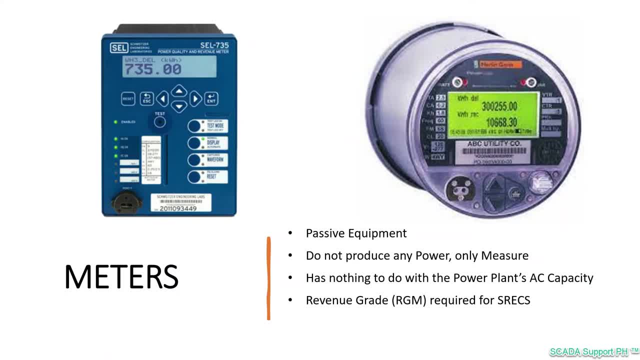 do is measure them, meaning you can place as much capacity or inverse behind the meter as needed as meters does not determine your ac capacity. all it does is measure the instantaneous power in kilowatts as well as the accumulated energy in kilowatt hours. measuring ac energy delivered by a pv system can be broken into main categories. 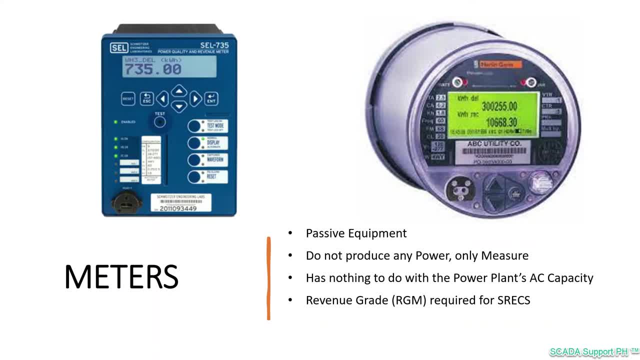 you have your revenue grade and a non revenue grade. a meter specified as being revenue grade is one that meets the requirements outline in the ansi standard c-12.1 of 2008, and and it is the one required for performance-based incentives, such as SRECs or your solar renewable energy certificates. 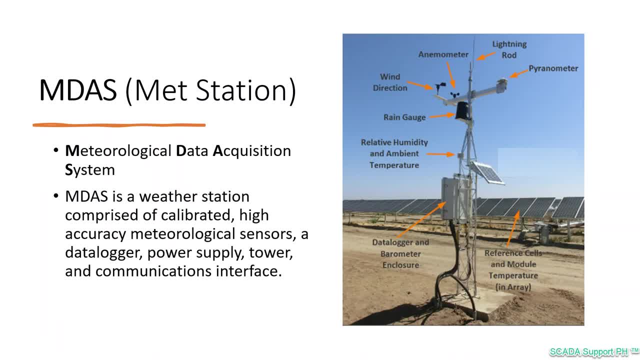 In this section, we will discuss the MET station. MET station is defined as a meteorological data acquisition system wherein you only need to measure your weather data. These include a pyranometer for measuring global horizontal erasions. You also have your wind sensor. 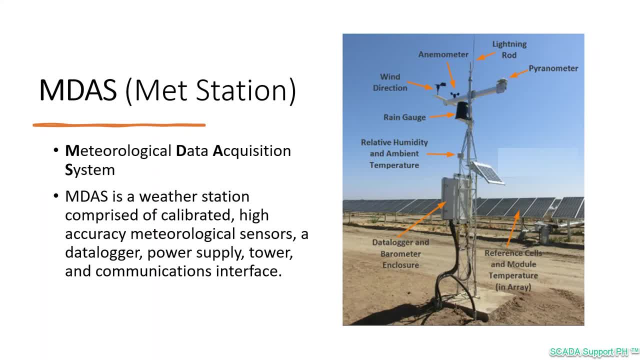 which includes wind vane and anemometer, rain gauge, ambient temperature, relative humidity sensors, as well as a barometer For sun tracking systems. we need to have a reference cell. These are just single cells that are mounted within the array. 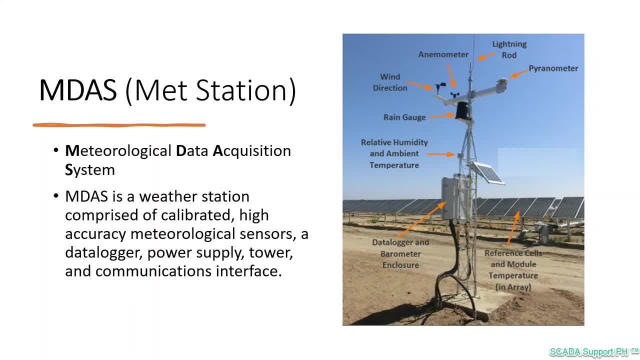 and it's being used for erasions measurements in line with the sun tracking system and not with the global horizontal erasions or GHI. We also have the back of module temperature sensor which are mounted in the array as module temperature affects the module's performance. 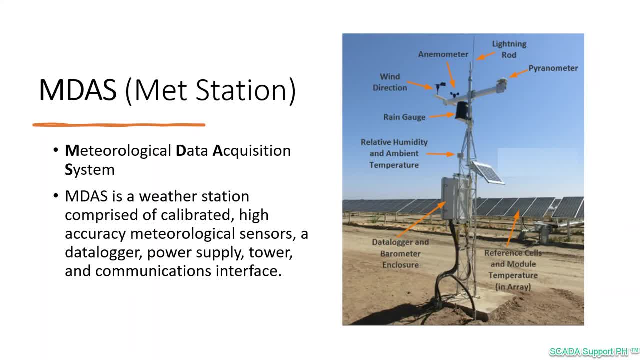 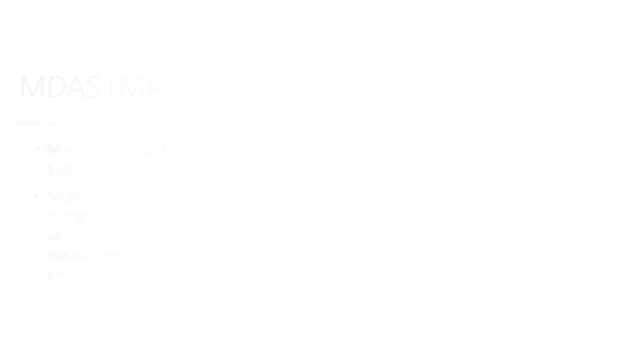 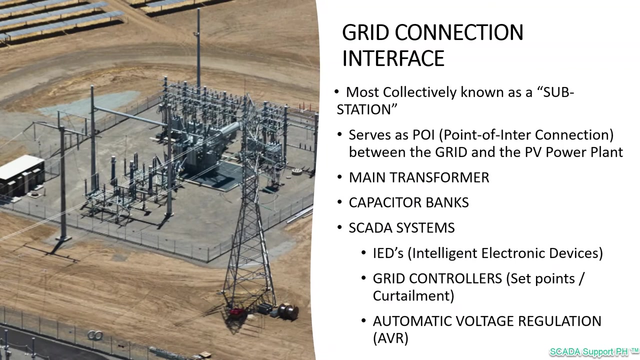 during operations. For all those weather data to be collected, you'd have a data logger that pulls data from those sensors and transmit them back into your SCADA system. For a PV power plant, we need to have a data logger that pulls data from those sensors and transmit them back into your SCADA system. 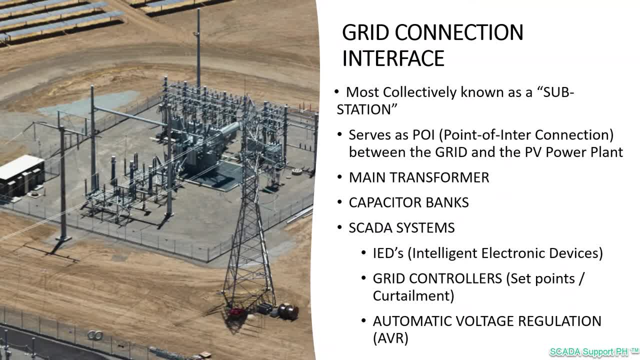 For a power plant. the substation serves as the grid connection interface, which is similar to a POI or point of interconnection between the grid and your power plant. this composed of your main transformer, capacitor banks and your SCADA systems. When we talk about step up transformers, 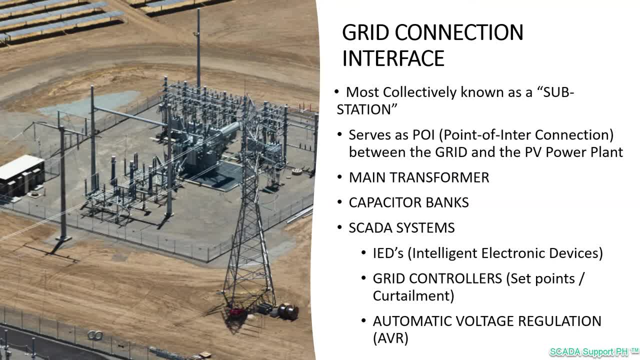 The output from the inverse generally requires a further step up in voltage to reach the AC grid voltage levels. The step-up transformer takes the output from the inverse to the required grid voltage, like for example, 25 kV, 33,, 38, or even 110 kV. 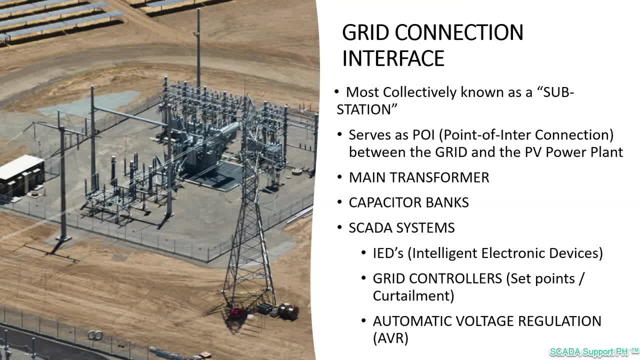 depending on the grid, connection point and country standards. We also need to have grid controllers that accept commands or set points from the grid or the utility if there are needs for curtailment or change the power factor in a given instance, and eventually apply them to your PV system. 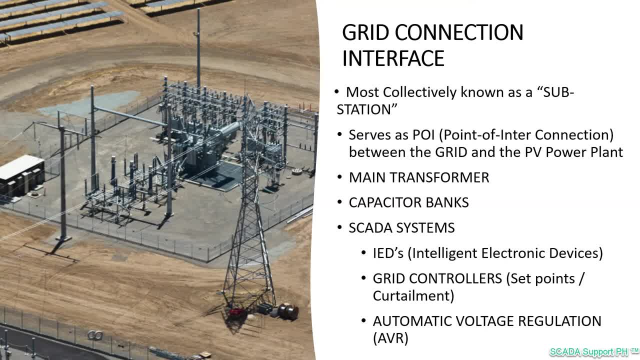 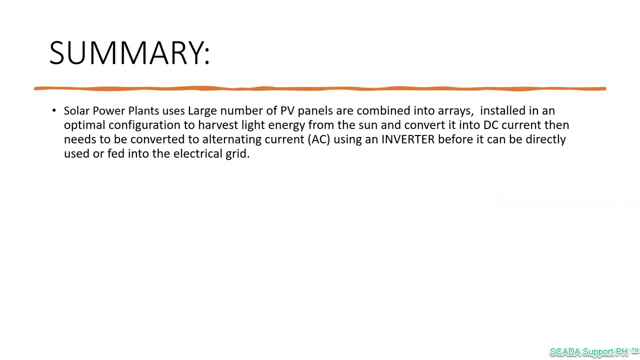 If you need to know more about SCADA systems for PV plants, please check the other presentation in the links below. They should be available at the top As a summary. solar power plants uses large number of PV panels that are combined into arrays. 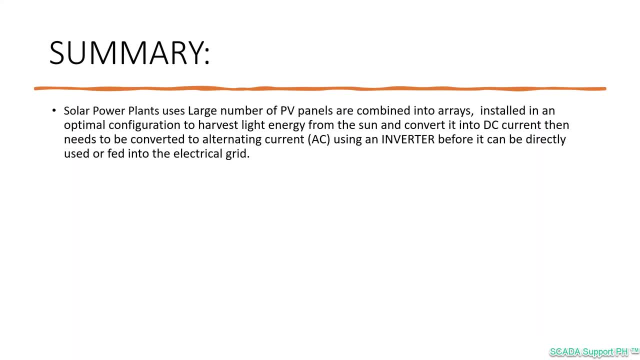 installed in an optimal configuration to harvest light from the Sun and convert it into DC current, and your inverters use to convert them to AC current. before it can be directly used or fed into the electrical grid, The output power of a power plant should be greater than 1 megawatt and 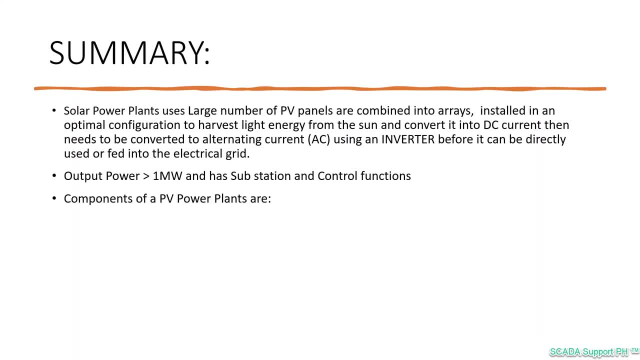 you need to have a substation and control functions. The components of a PV power plants are solar array mounting systems, wiring, skid or pads, grid controller interfaces in which you have your main transformers, your SCADA system and controllers that are usually located within the substation. 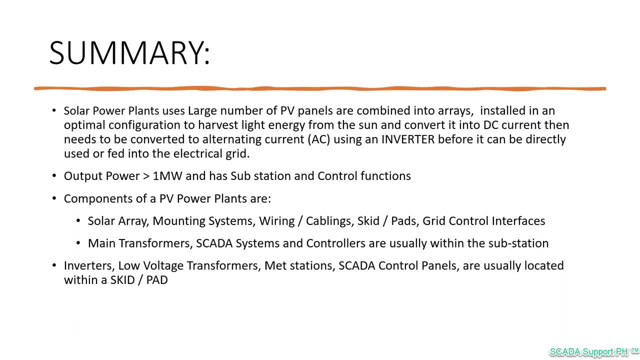 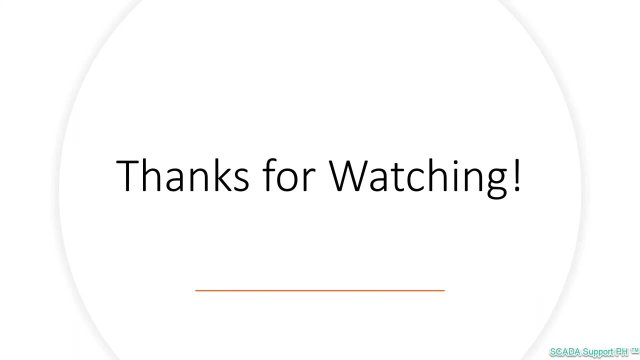 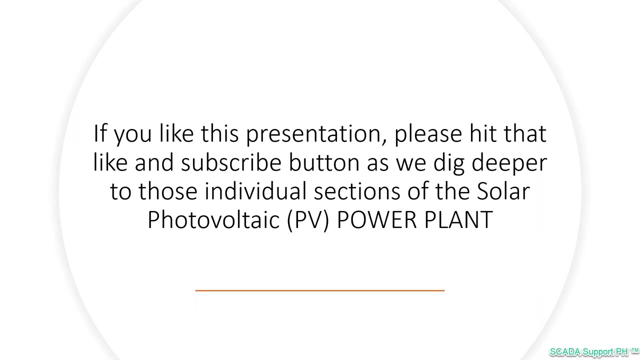 Inverters, low voltage transformers, MET stations, SCADA control panels are usually located within the substation. The power plant substation serves as your grid connection interface. That's all for now. Thanks for watching. If you liked this presentation, please hit that like and subscribe button as we dig deeper to those individual sections of the solar PV power plant. Thank you. 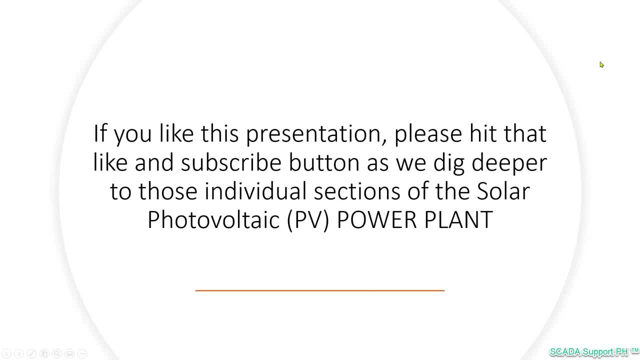 If you have any questions or other problems, please post them in the comments below. If you have any questions or other problems, please post them in the comments below.